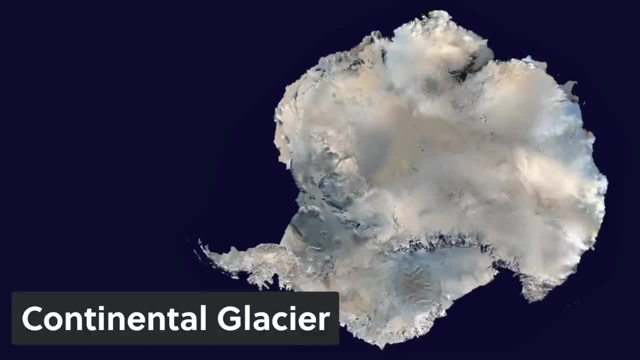 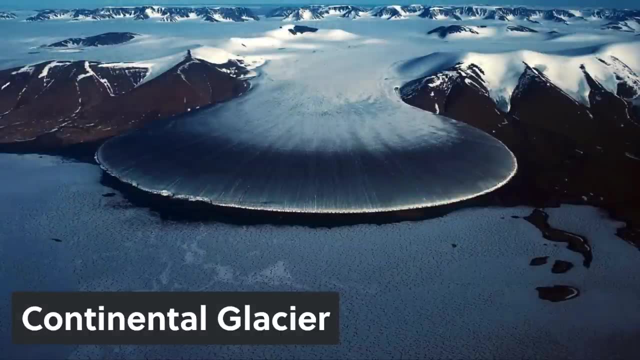 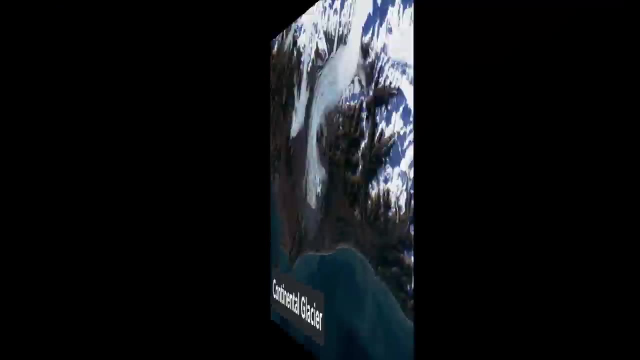 largest glacier in the world. It has a huge thick sheet of ice that covers virtually the entire land mass. We see a similar thing in Greenland. Up close you can see these huge sheets of ice ooze out from the center towards the coastline, slowly grinding away the rock beneath. When 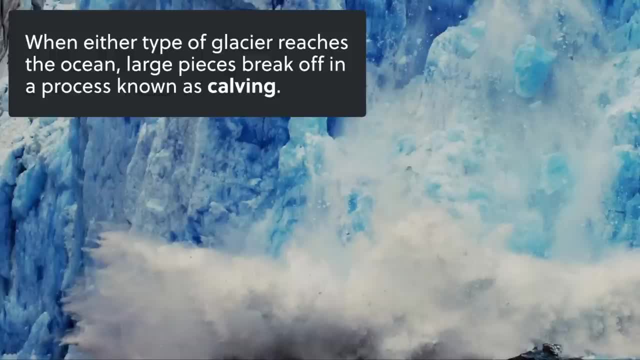 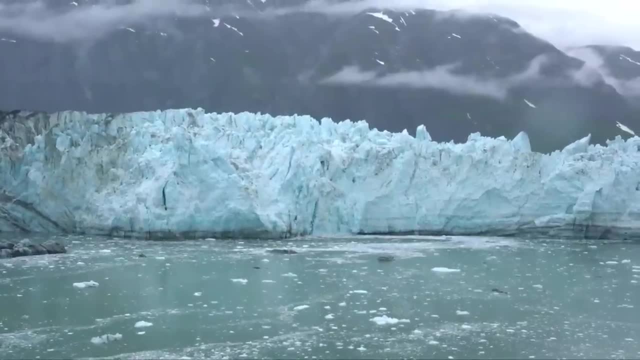 either type of glacier, whether it be alpine or continental. when they reach the ocean, large chunks of the ice tend to break off, and this is a process that's known as calving, And you can see it happening here As climate change continues and the atmosphere and oceans. 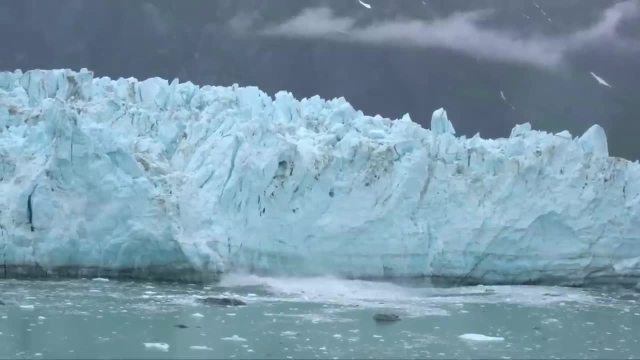 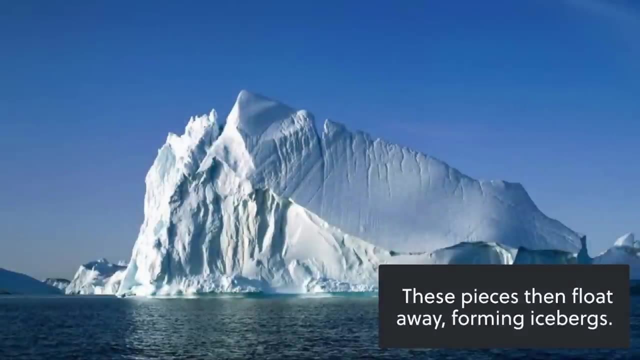 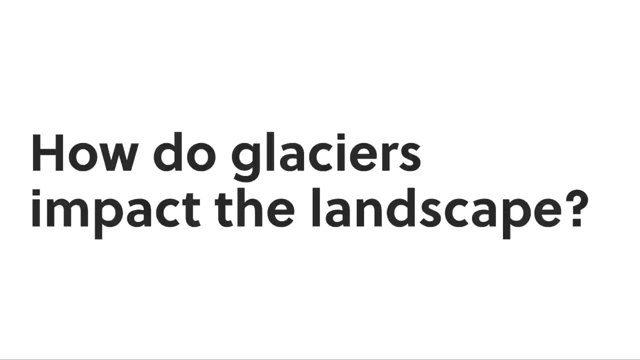 are warmed, calving is happening at a faster rate. These big chunks that fall off of the glaciers then float out into the sea, becoming icebergs. The most important thing to look at with glaciers is how they impact the landscape, That is, how do they change the land as they grind over the. 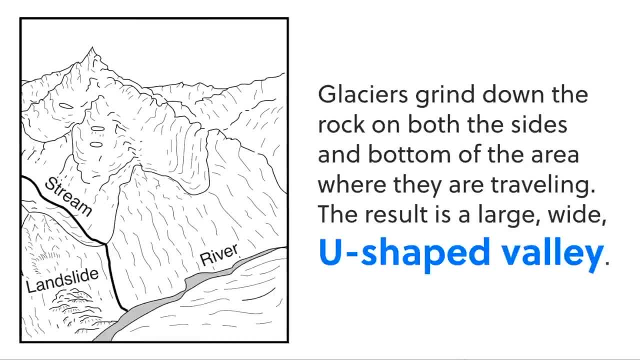 surface over millions of kilometers of land. This is a very important question. The question is: how do they change the land as they grind over the surface over millions of kilometers of land? First and foremost, we should know that glaciers grind down the rock that's on both sides and on 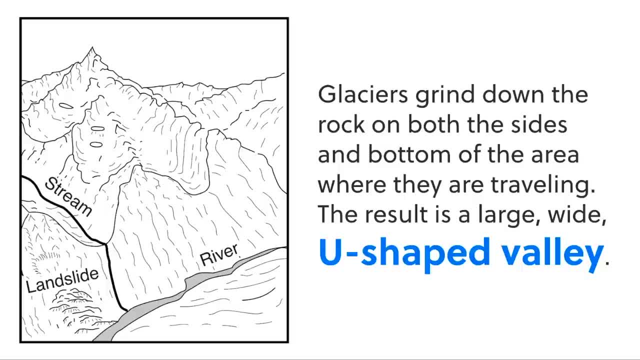 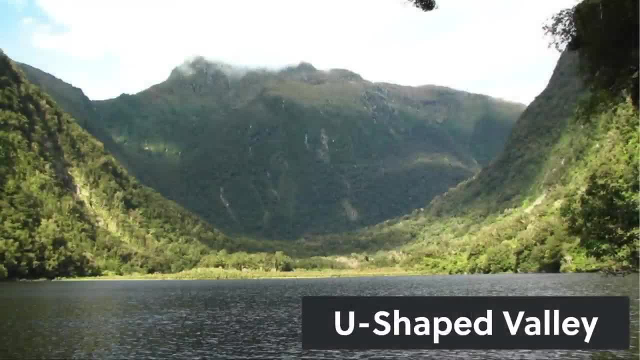 the bottom of the area where they're moving, and the result is this large U-shaped valley which you can see here in the diagram. Notice it's shaped like the letter U. Here's what it looks like in reality. We can infer that this valley was formed by glaciation at some point. 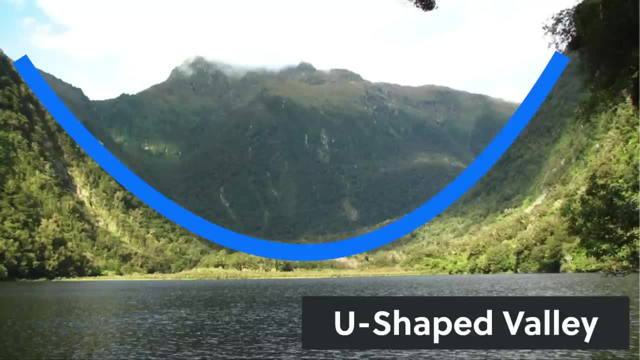 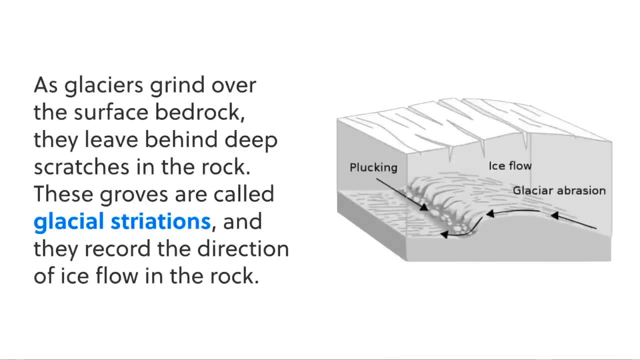 in the past, and that inference is based on the general shape of the valley. Here's another U-shaped valley. As glaciers grind over the bedrock, they scratch it. They leave behind marks and grooves that are called striations, And these striations are important because they reveal the direction. 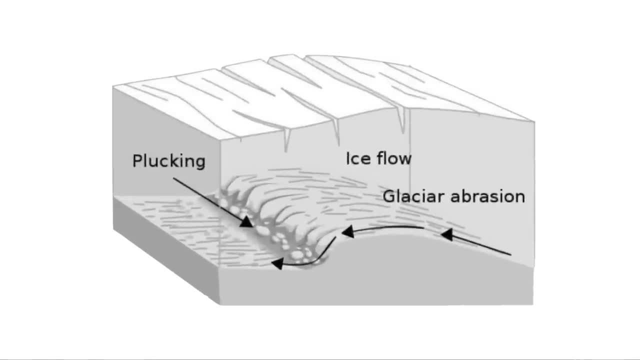 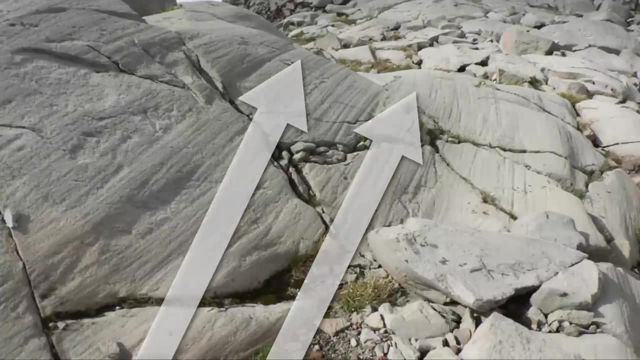 that the ice was moving before it melted. You can see them plucking and grinding away at the rock beneath, resulting in something like this, And by looking at those striations we can draw an inference about what direction the ice was moving. You can see that the ice was moving in the direction. 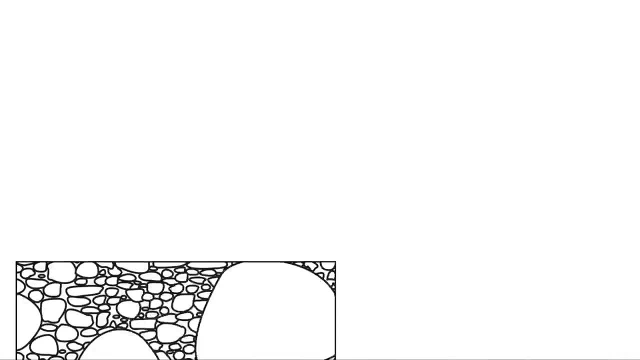 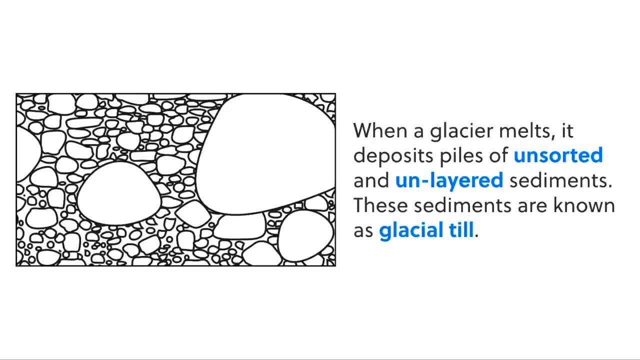 it was moving. We see them here as well. When a glacier melts, it's going to deposit or drop off all of the sediment, all of the pieces of rock and sand and silt and clay that it was carrying with it, And when it does so, it just kind of drops it off, And so we end up with these big 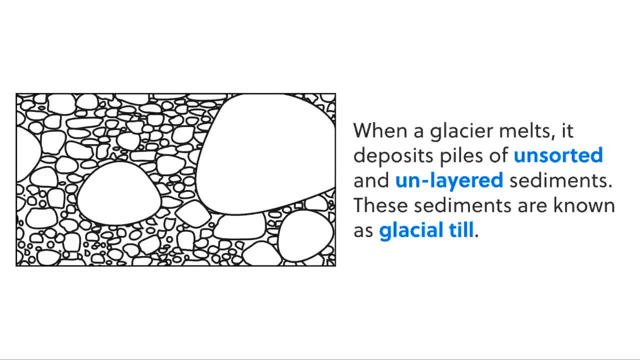 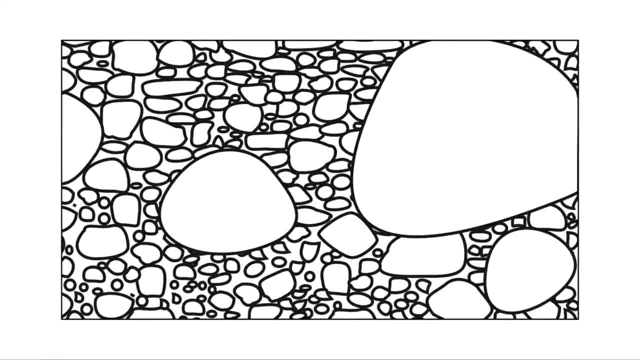 piles of this unsorted and unlayered sediment, And we have a term for these sediments and that's called glacial till. Here you can see big, small all mixed together, And this is what it looks like in reality, And this serves as further evidence that there 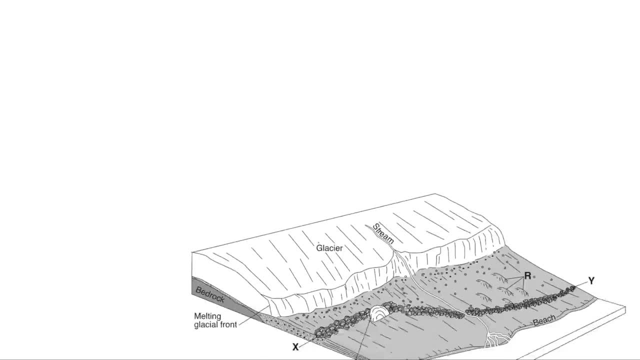 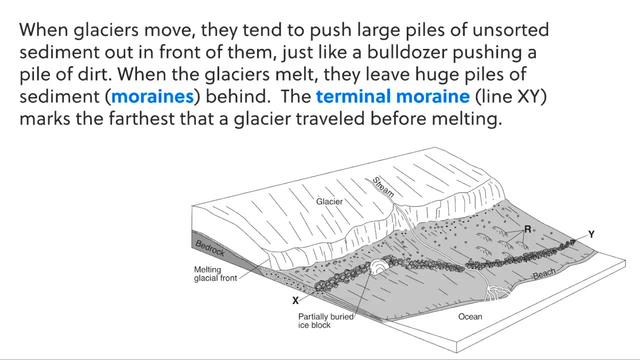 was once a glacier in this area. When the glaciers move, they push this till or this unsorted sediment out in front of them, very similar to a bulldozer pushing a pile of soil. When the glaciers then melt, they leave behind these piles of sediment, And these are called. 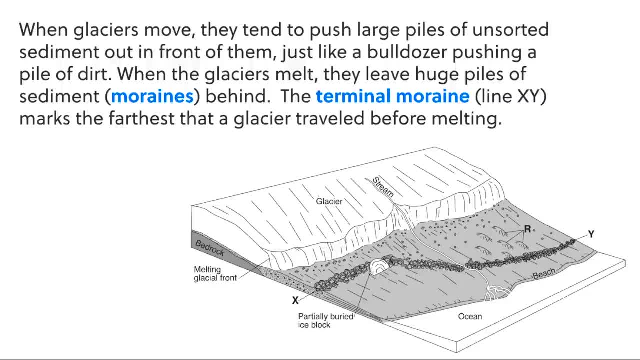 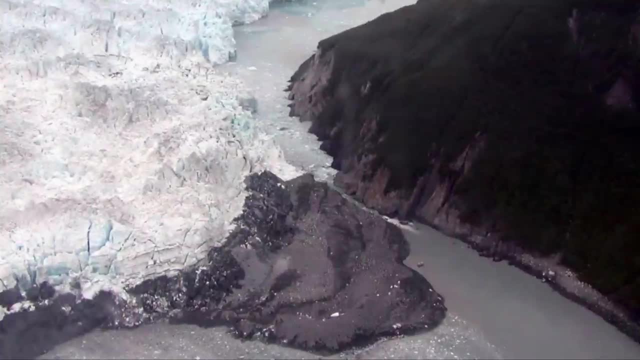 moraines. Moraines reveal a lot about a glacier, particularly the terminal moraine shown in this diagram, line XY. This marks the farthest point that a glacier traveled before it receded or melted away. Here's a terminal moraine. in reality, This area right here is the. 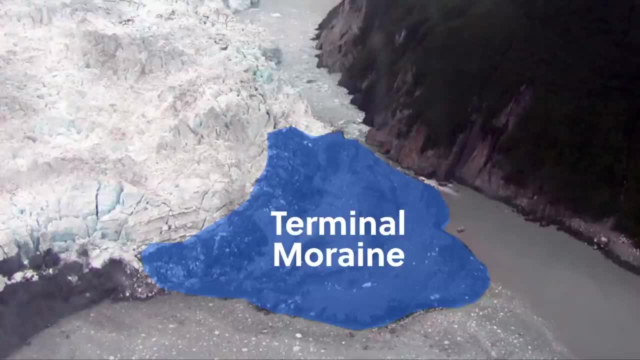 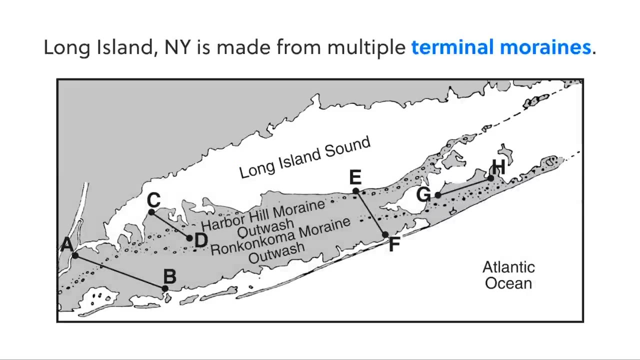 till the unsorted, unlayered sediment that was pushed out in front of the glacier. We can see another terminal moraine right here. Long Island, New York, is a great example. It is formed as a period of glaciation And therefore there are multiple terminal moraines: The Harbor Hill. 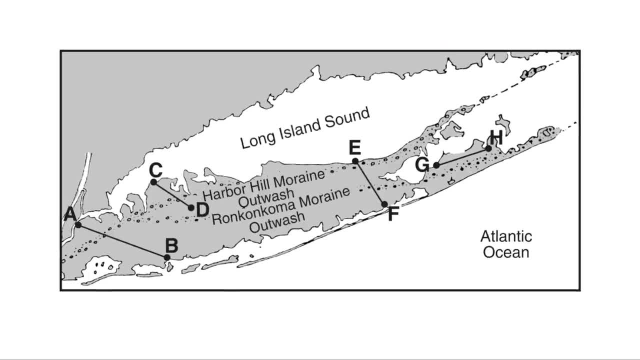 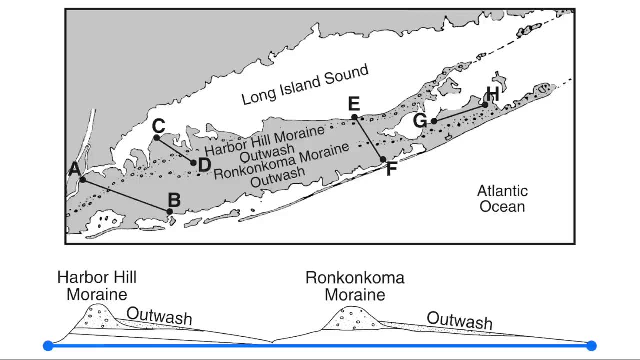 moraine, the Ronkonkoma moraine, etc. If we were to look at line EF here from the side as a profile, it would look like this: You would have this first moraine And then notice this term outwash. 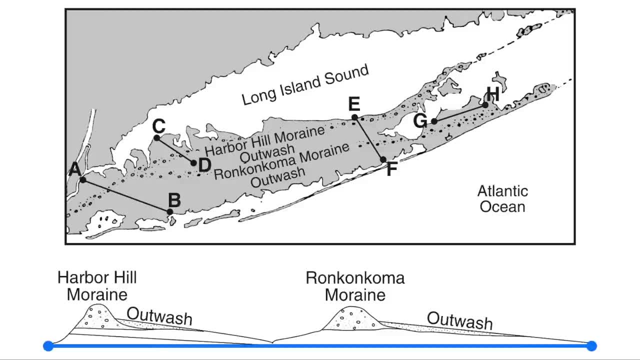 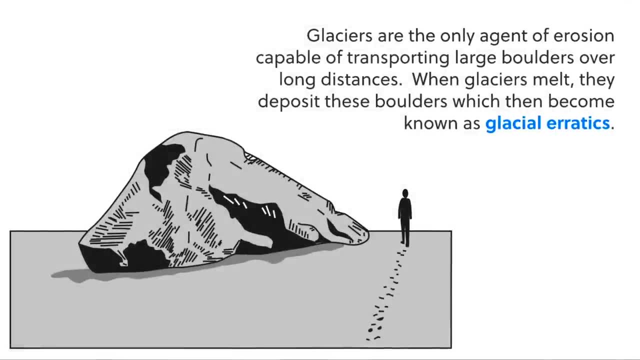 which is just some of the material that's been washed out by melting water. And then we have a second period of glaciation that resulted in the Ronkonkoma. moraine Glaciers are the only agent of erosion that are really good for the environment, And that's what we're going to talk about today. 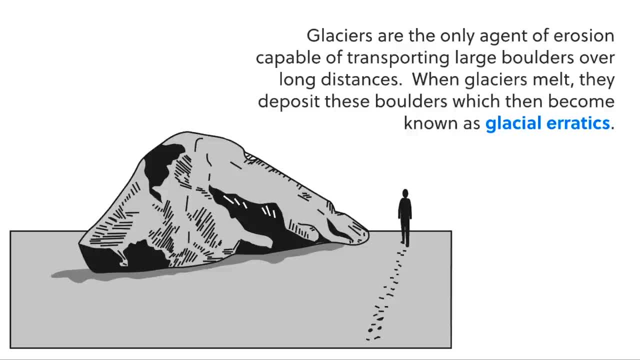 Glaciers are really capable of moving large, large boulders. These are called glacial erratics. So when we see randomly scattered boulders throughout the landscape, we can infer that they were moved there by a glacier, And that's because running water or wind are not capable. 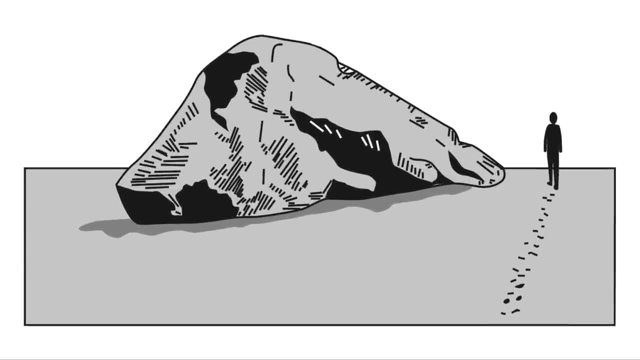 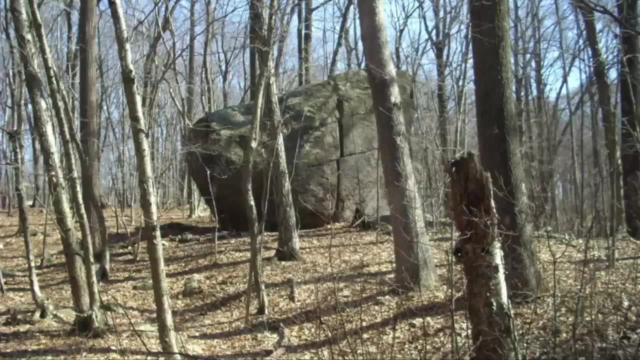 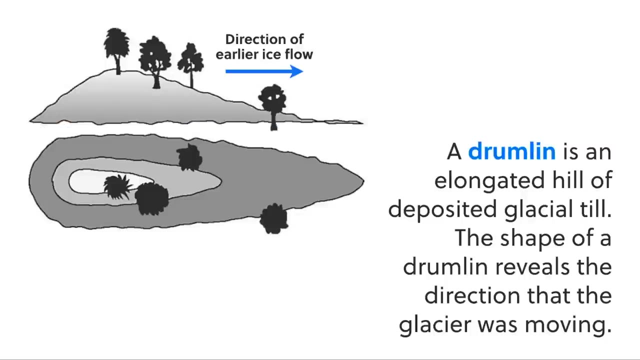 of moving such large sediments. Here's a glacial erratic And here's what they look like in reality. The only way these sediments could have gotten there is by being transported by a glacier frozen on the edge of very large sheet of ice. Oftentimes, glaciers will leave behind something called a. 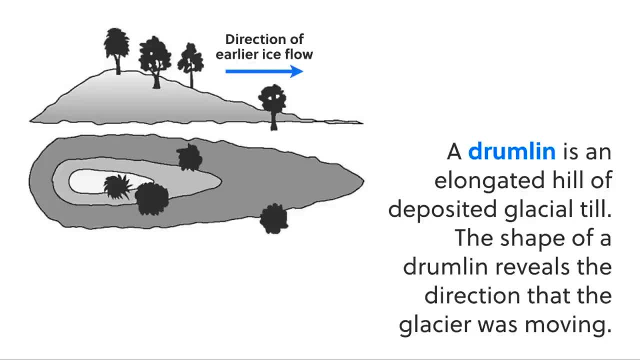 drumline, which is simply an elongated hill of sediment. Remember the sediment would be unsorted and unlayered. What's interesting about drumlines is the shape that they often take as the ice goes up and over and moves the sediment, You end up with this teardrop shaped hill, And by looking at the 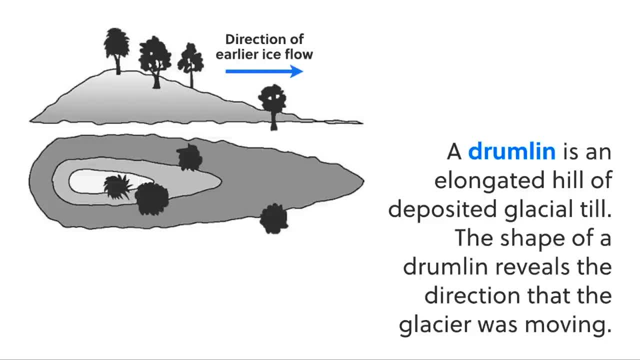 shape of the hill, you can determine the direction that the ice flowed. It often flowed towards the flatter side of the hill- a little great- as well as the pearly side of the hill. It's also able to float, dizzy, Go, brush or wrestle in the distance and take rest in your great as well. You don't have to. 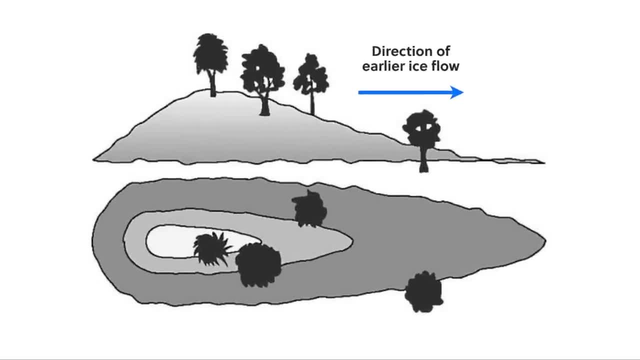 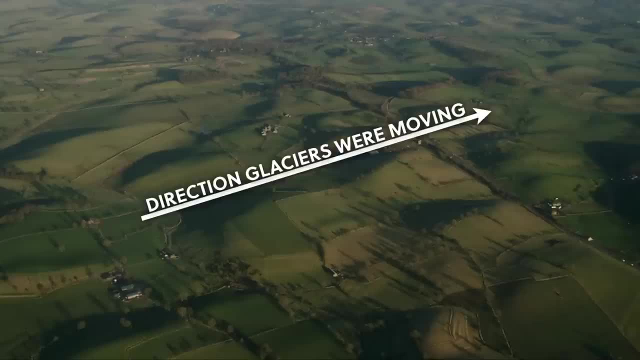 even think about going table to table with vast amounts of ice on each kosher makes great granite in my life. of the hill, the less steep side, Here's a field of drumlins in upstate New York and by looking at the shapes we can tell that the ice was moving in this. 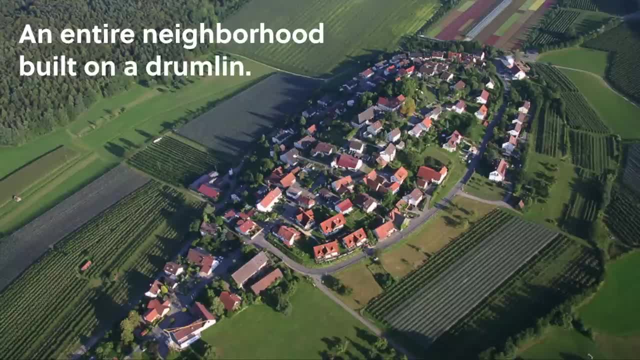 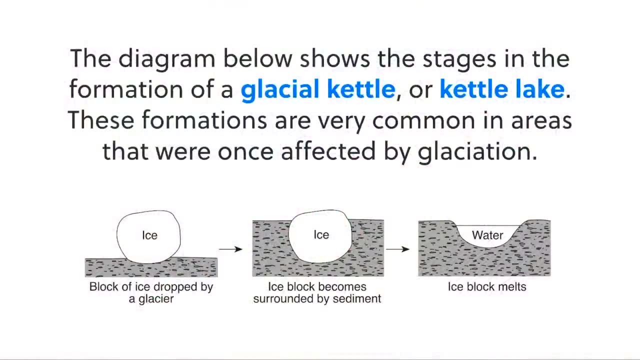 direction. Here's an entire community that appears to have been built right on top of a drumlin, surrounded by farming fields. This diagram shows us the stages in the formation of what's called a kettle or a kettle lake, and this is very common in areas where you've had glaciers. What happens is large pieces. 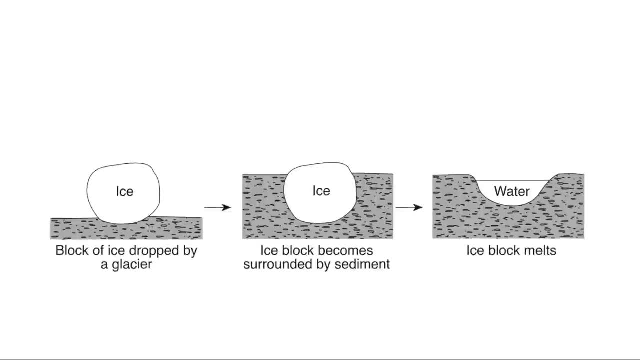 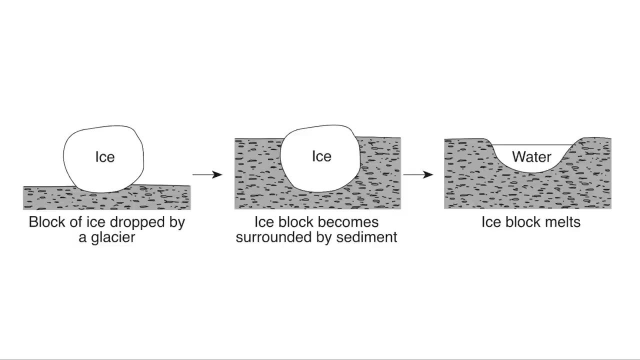 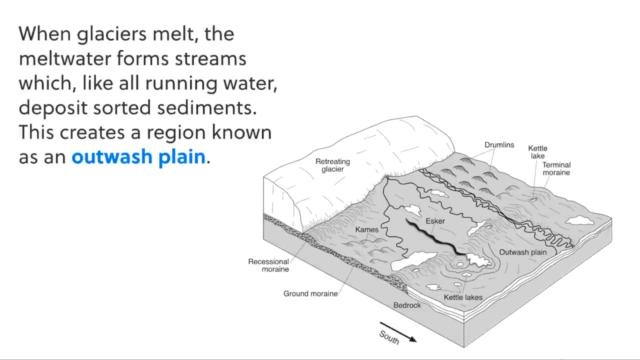 of ice break off from the glacier, and then that ice gets buried by some sediment and then eventually melts, leaving behind a hole in the ground known as a kettle, and if it fills with meltwater it'll be a kettle lake, as seen here and here. When the glaciers melt, we get a lot of meltwater, which forms 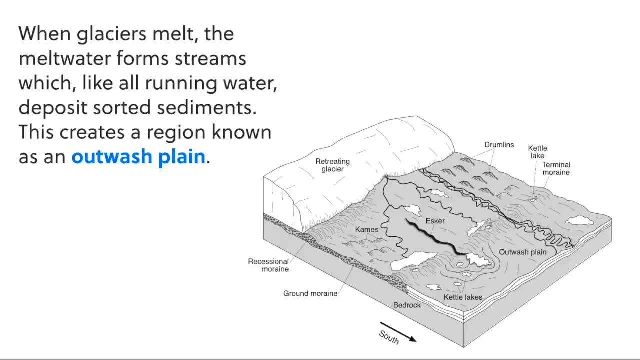 streams coming off the front end of the glacier. Like all running water, these deposit sordid sediments. So remember, the sediments deposited by the glacier itself are unsorted. that's our till, creating our moraines. but when we have outwash, when we have water, that's become liquid and 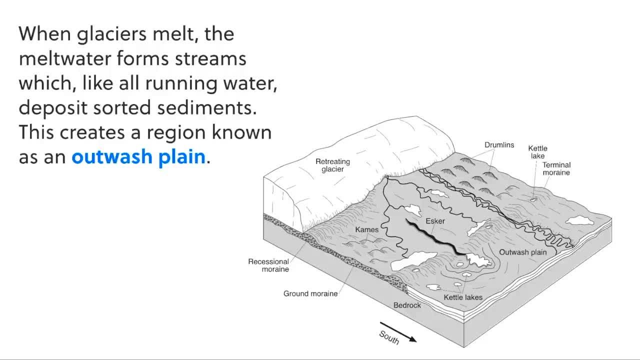 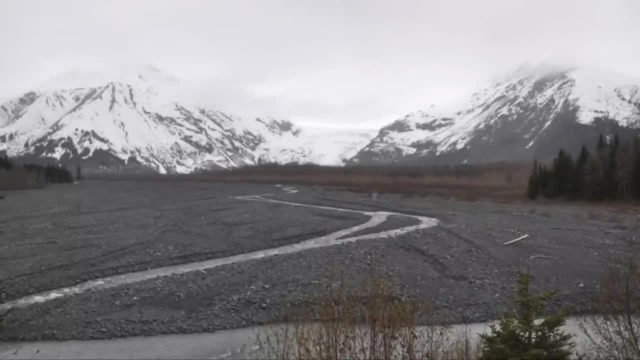 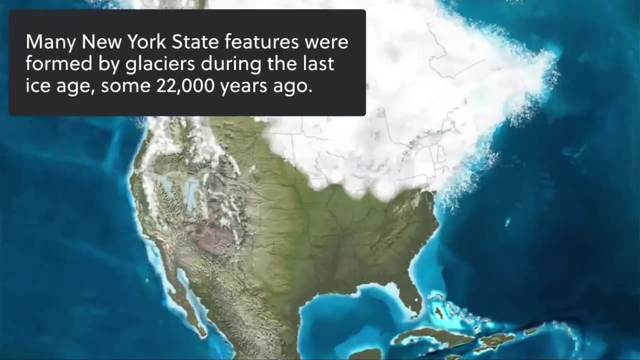 melted, creating streams. then we end up with some sordid sediments and you can see that in this diagram here This is an outwash plane. so all of these sediments were deposited by runoff from melting glaciers, also seen here If we look at.